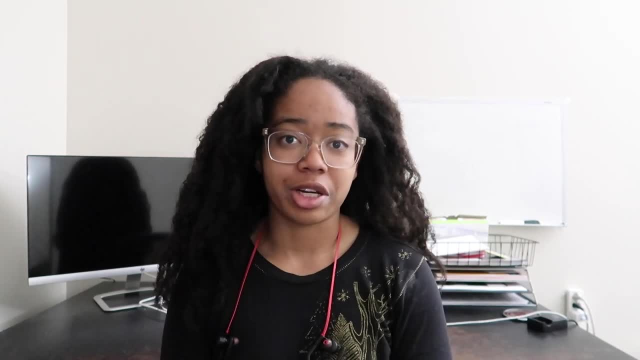 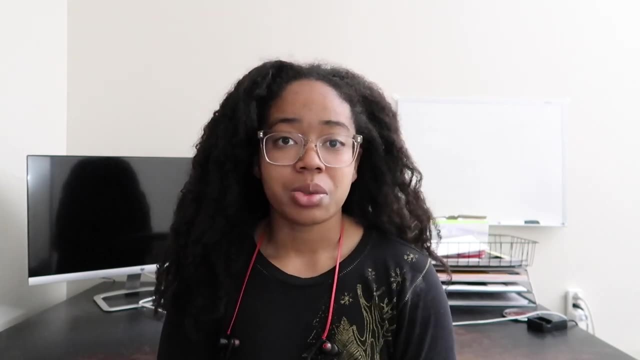 school and I liked it. I liked programming. We were learning in Java. For me, programming is kind of another language that I can use to speak to, in this case machines. So as an undergrad I went to Cornell and I was interested in engineering. 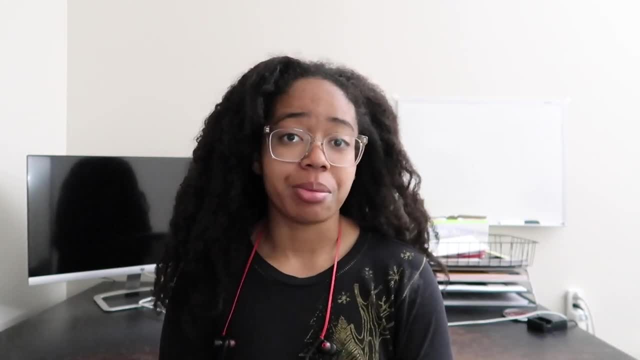 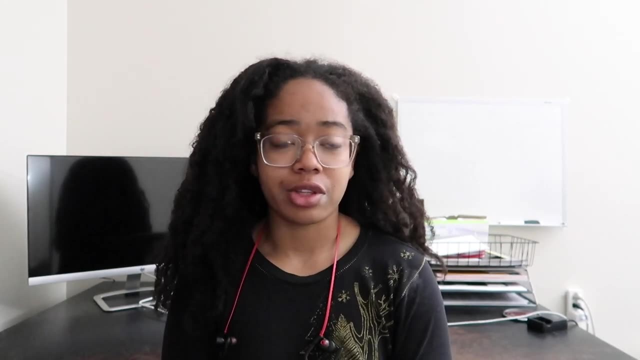 But I wasn't sure what kind I'd done research in high school in biomaterials. but Cornell didn't have an undergrad in biomedical engineering when I applied, so I figured that I would do some other major, maybe electrical engineering or material science, and then figure out a way to do research. 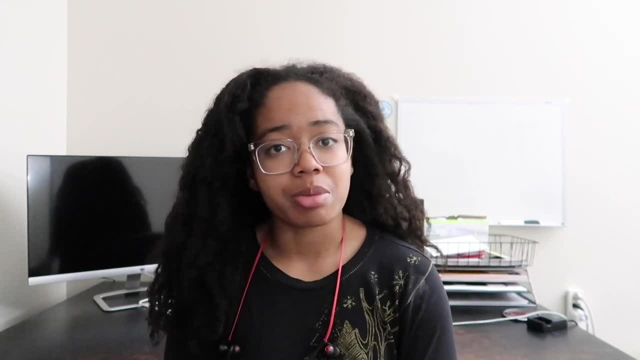 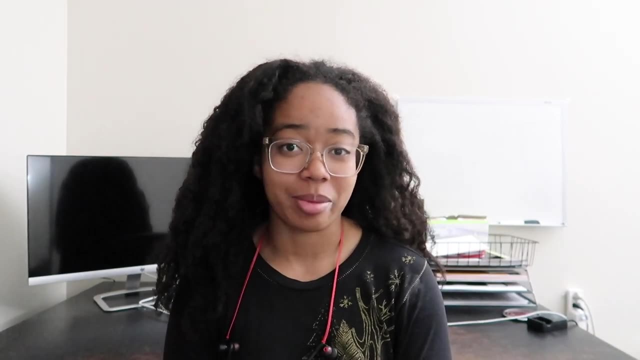 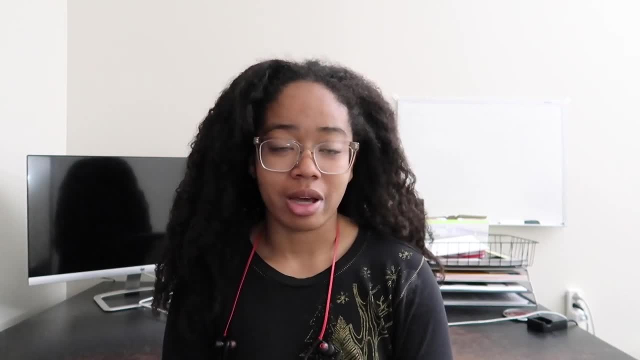 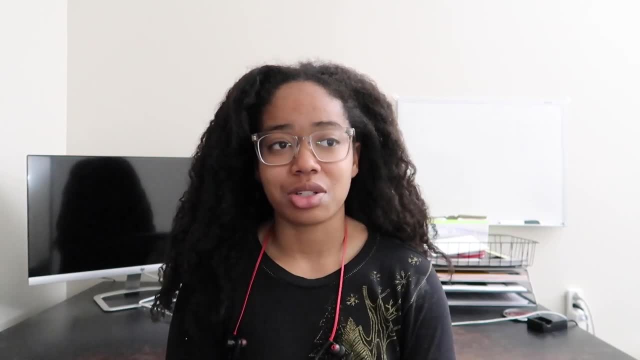 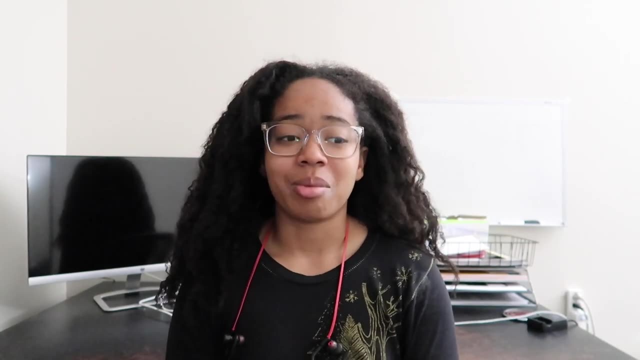 that major. One of the benefits of being in the first class is that Cornell has these distribution requirements and there's usually electives within your major, And so since we were first, we kind of got to pick what we wanted. There wasn't really a formal list yet, And so that let me kind of shape. 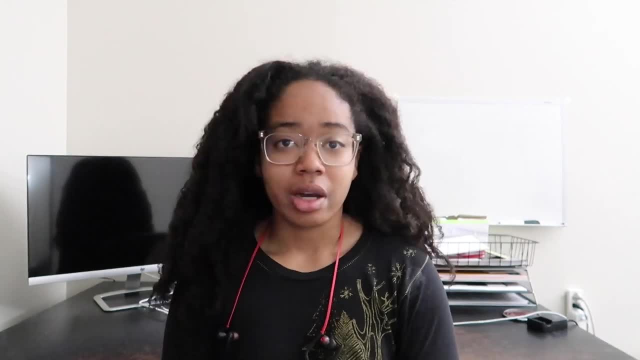 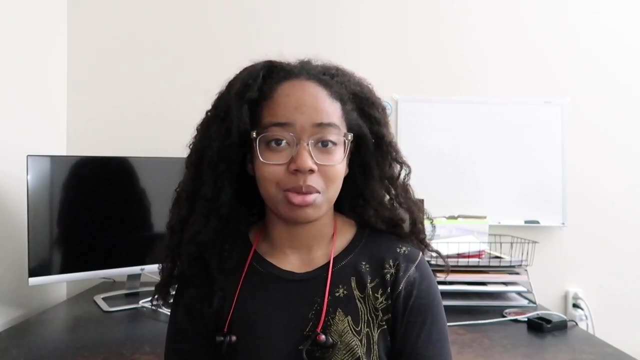 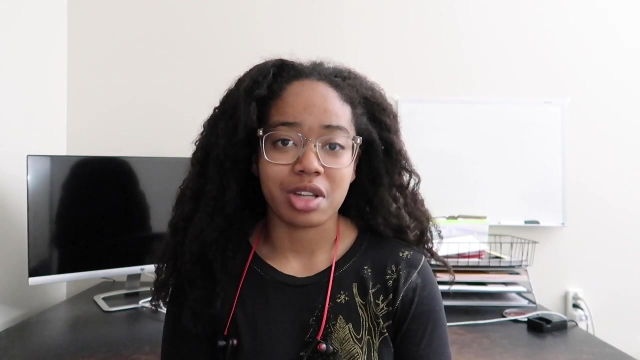 my program towards the things that I was interested in. Now I mentioned. I joined a lab over that first summer and I actually spent three years in a cartilage engineering lab, so nothing to do with machine learning. I was working with biomaterials and material science, looking at ways to engineer. 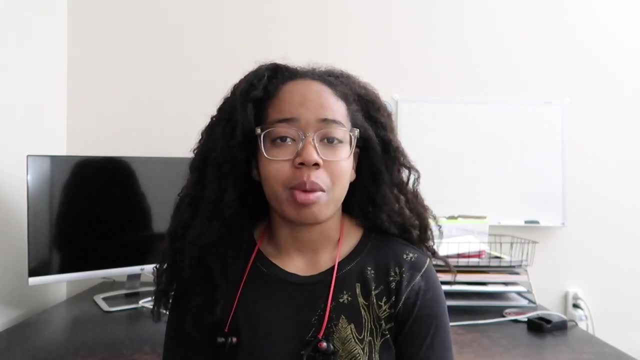 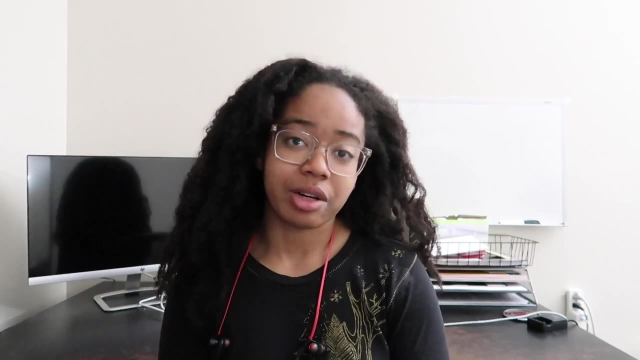 the meniscus which is in your knee. Somewhere. during my sophomore year, I think, I realized that I was more interested in the data analysis that I'd been doing. We were using CT images, which are kind of medical imaging, to analyze some of our samples. 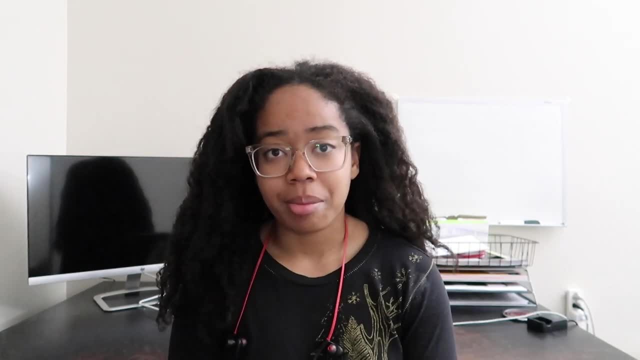 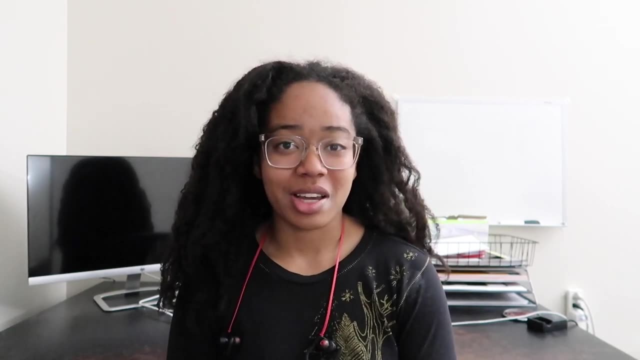 And I really enjoyed the analysis that I was doing in MATLAB, which was another language that I picked up thanks to Alex, the grad student that I worked with, who asked me what languages I knew how to use, which at that time was basically Java, and then told me to do it in MATLAB. So I 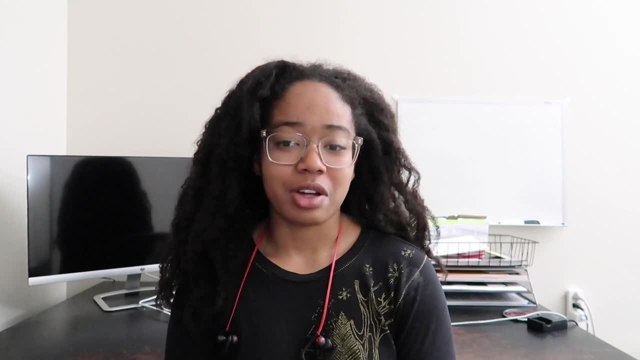 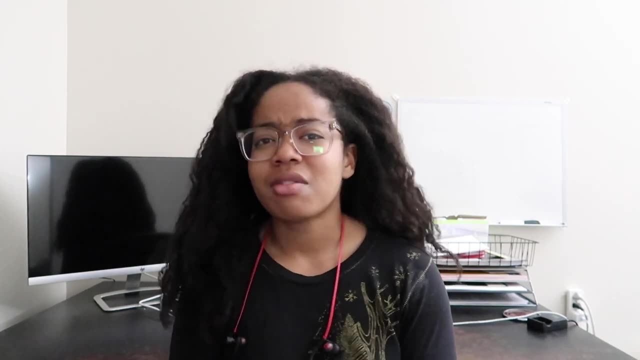 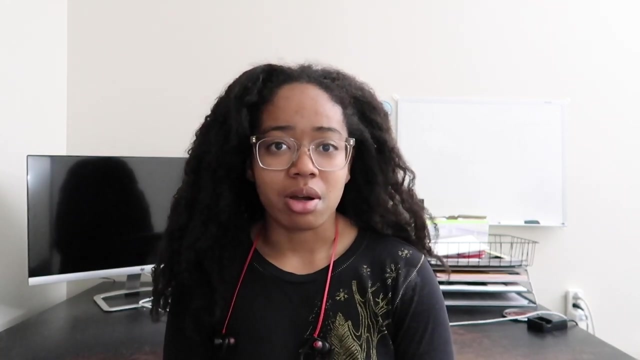 started taking more programming classes. The grad student that I worked with also realized pretty quickly that I was more interested in the computational end of things And we didn't have a ton of people in the lab doing that. So when I asked to kind of make that pivot, it was actually welcomed and I started doing a lot more kind of. 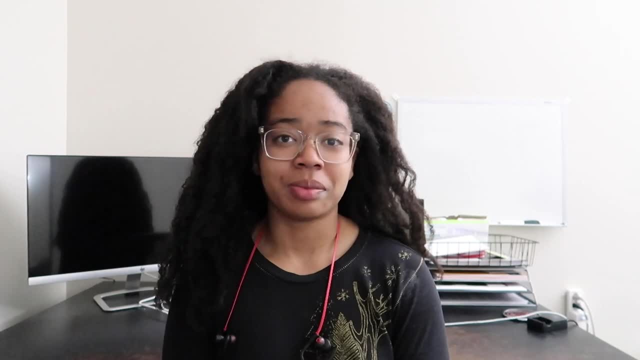 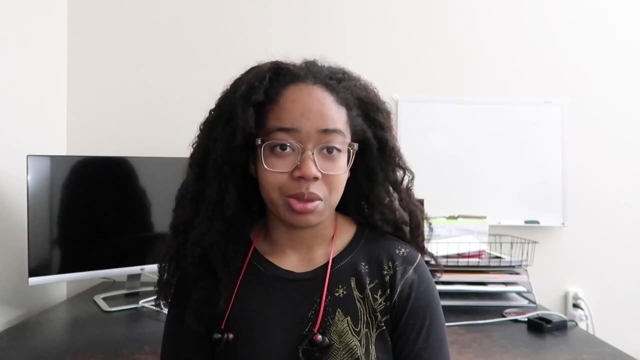 computational analysis, And, if it sounds like I'm being vague for those of you not familiar with the academic publishing system, we actually have a paper that we submitted to a journal which is under review, And so I can't really talk about the specifics. 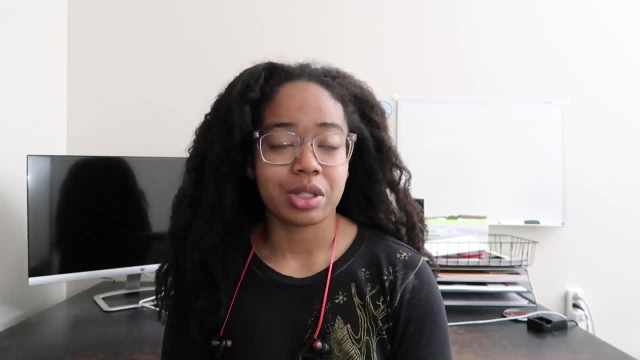 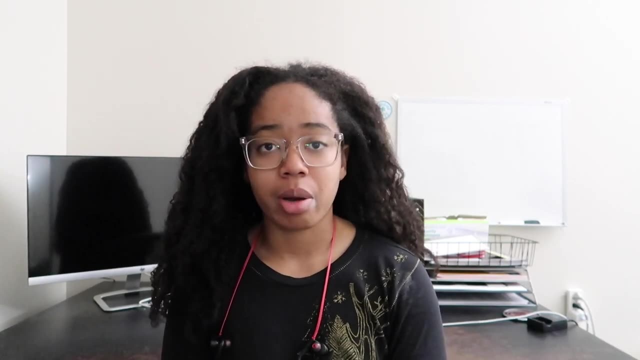 until it's published because it's not public work yet. So the summer after my sophomore year I kind of pursued that computational and medical imaging path a little bit more. I worked at Novartis with their clinical and translational imaging group on a bunch of different data analysis. 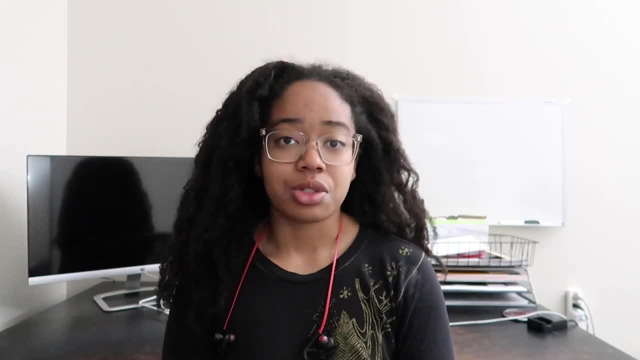 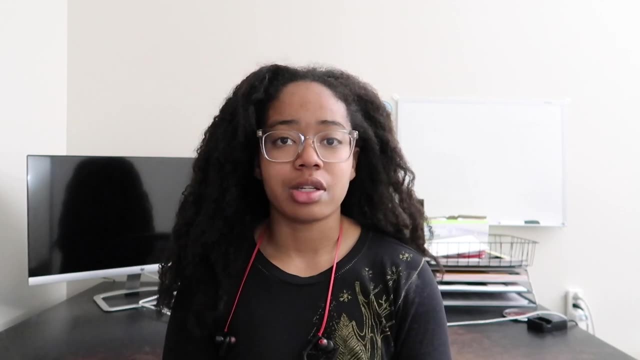 relating to preclinical trials and clinical trials. I was doing software validation for an external company that was looking to partner with Novartis, And so I think that that really helped me realize that I was still really interested in data analysis and computation, but I wasn't interested in it. 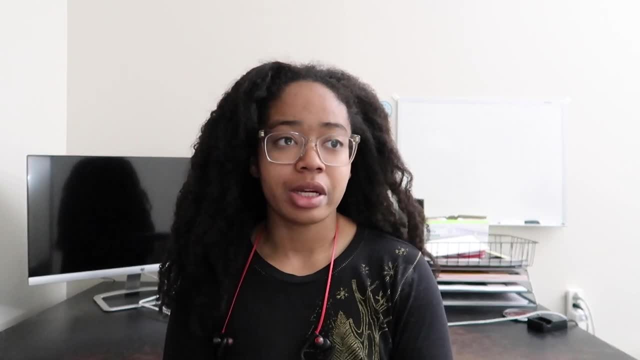 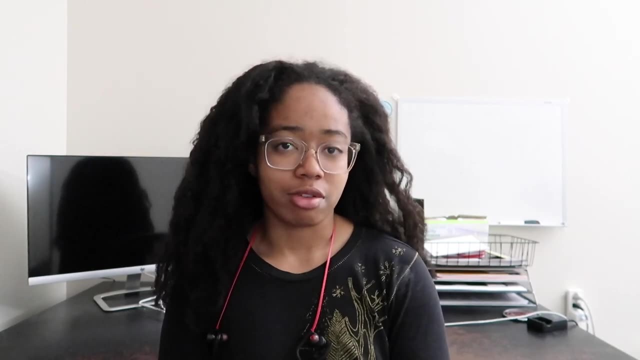 in industry, At least not at the entry level. For me. I really enjoyed having that intellectual ownership that you get in academia, where you kind of have your project and you work on all different facets of it, And so some parts of it may be computational and some parts of it might not be, but it's all. 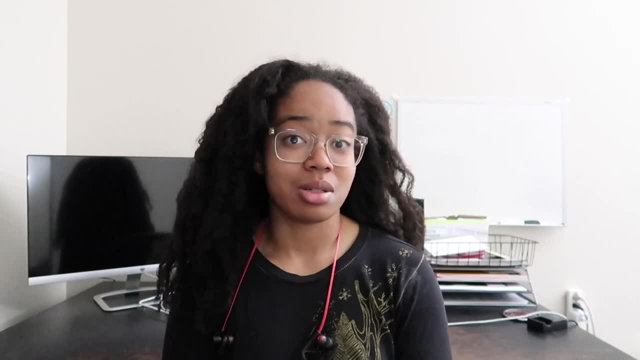 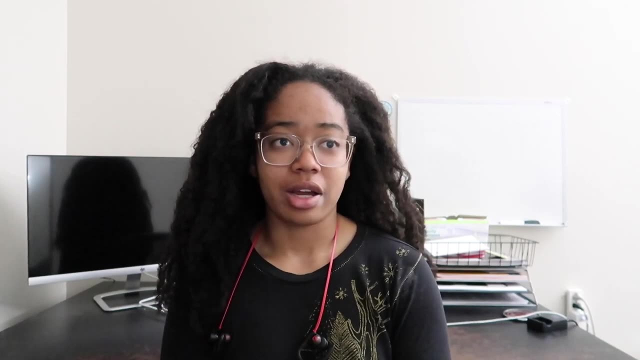 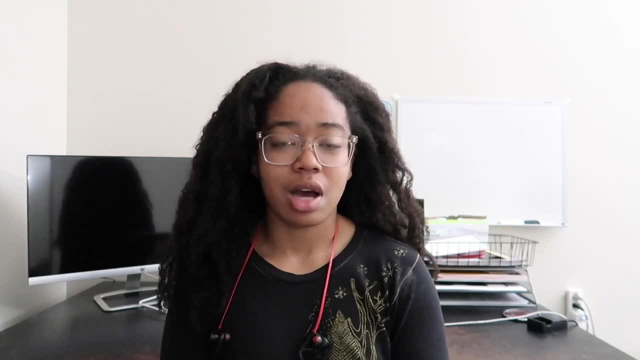 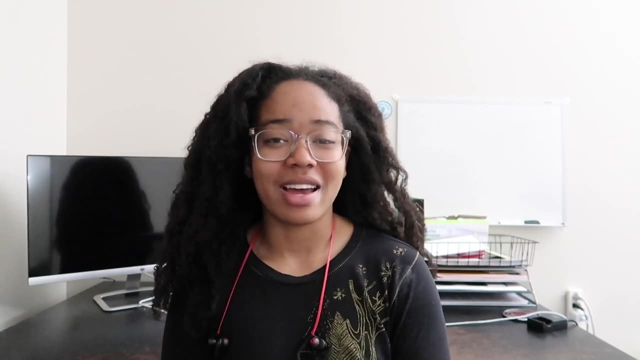 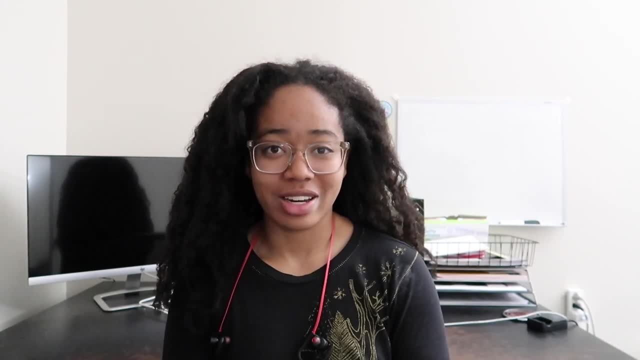 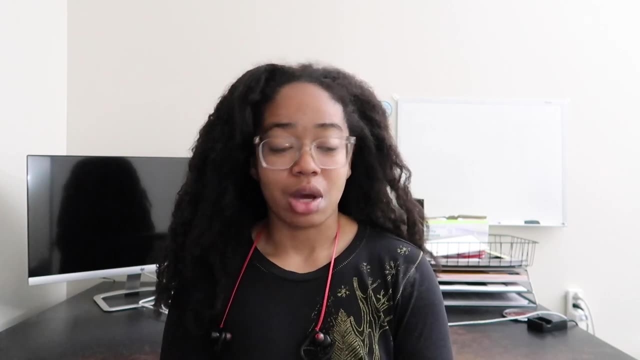 definitely a cool looking project, but I had no background in machine learning, And so that was really where I started to learn. So in the two weeks between getting my assignment and going to Stanford, I actually took Andrew Nigg's Coursera course. 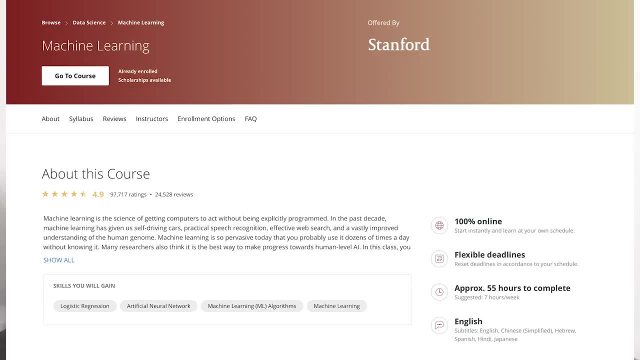 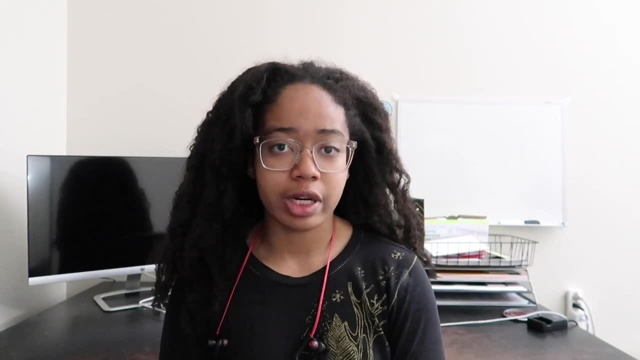 on machine learning learning, and I'll put a screenshot here or put a link in the description box. So I spent that summer at Stanford looking at MRI reconstruction using machine learning. We ended up submitting a paper to a workshop at Neural Ips, which is one. 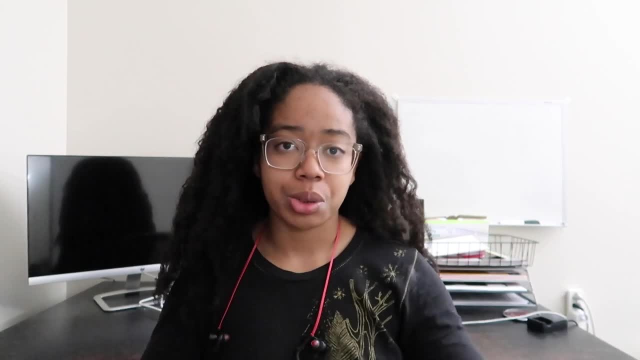 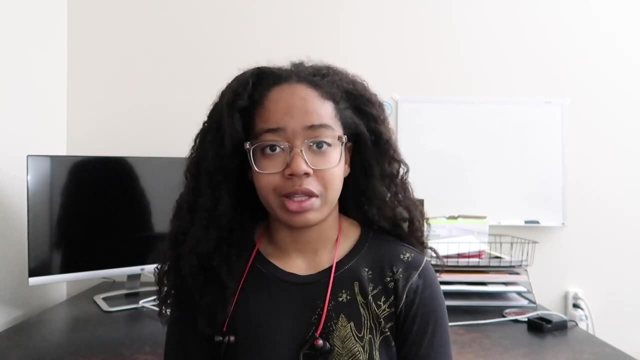 of the big machine learning conferences. I'll include a link to it below. but essentially what we were trying to do is look at MRI reconstruction and fixing errors in real time. I then spent the next year, my senior year of undergrad, picking up some smaller projects. So I took a neural engineering class where we 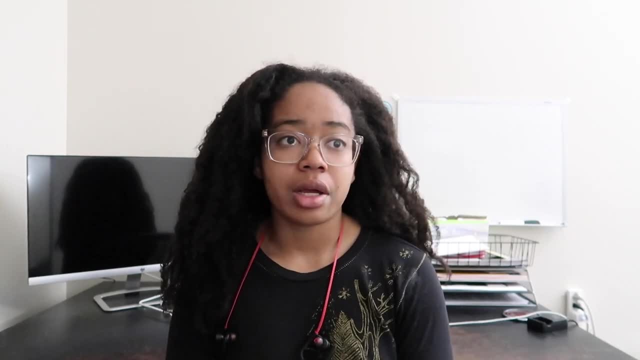 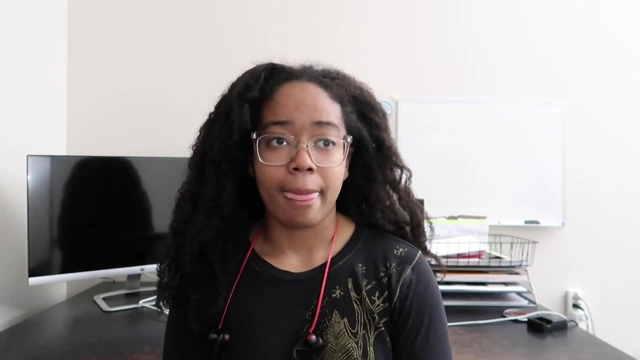 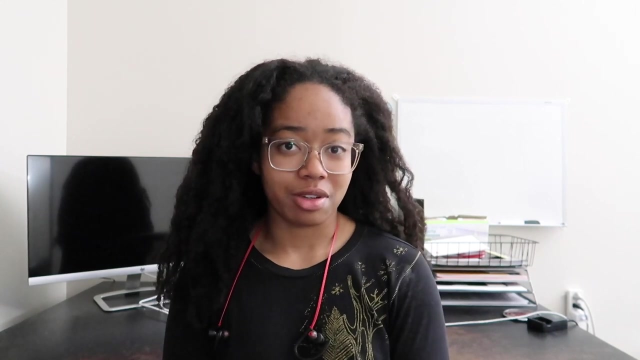 had to do epilepsy classification and then I was also applying to grad school. So I was applying to electrical engineering and biomedical engineering PhD programs and I ended up going here. So my program is the PhD program in medical engineering and medical physics, which sounds super broad because it is 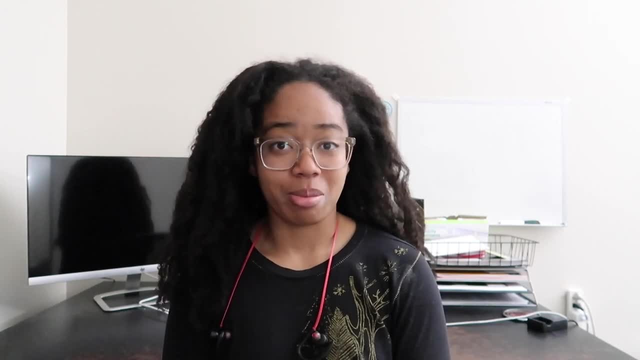 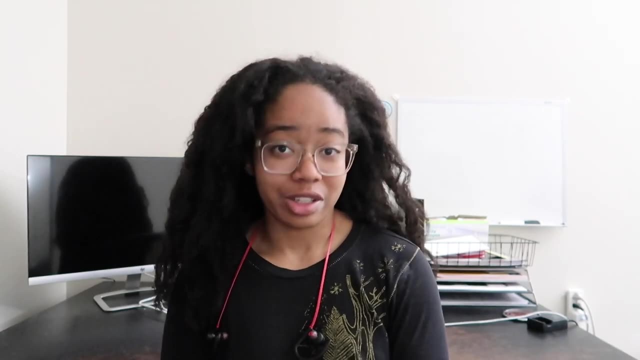 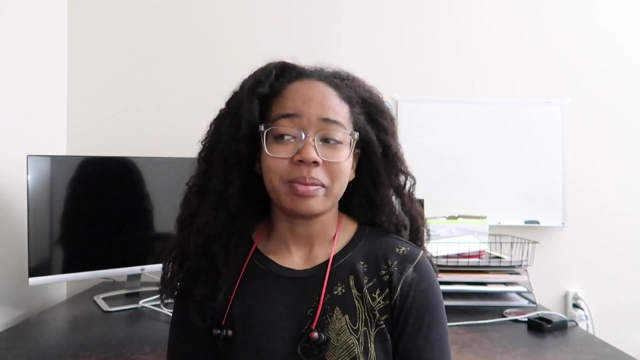 It's run through MIA T and Harvard Medical School. The overall, I guess, goal of our program is to teach PhD students to think like clinicians. So because of that we take all these MD classes. I had to do an autopsy last semester and the idea is to kind of put. 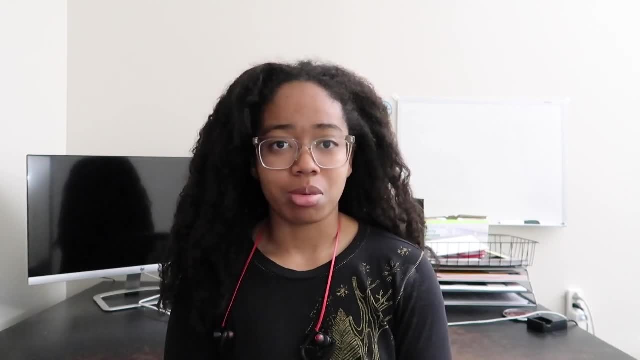 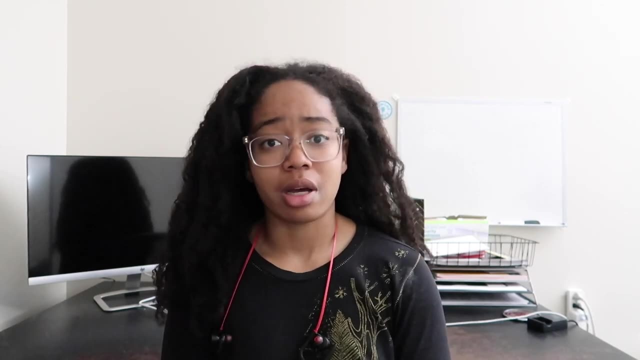 us in the clinic see what it's really like, so that we can solve real problems that occur in the clinic and see real problems that people who work on engineering problems for medicine may not otherwise be aware of because they're just not in the room when it happens. So I got to grad. 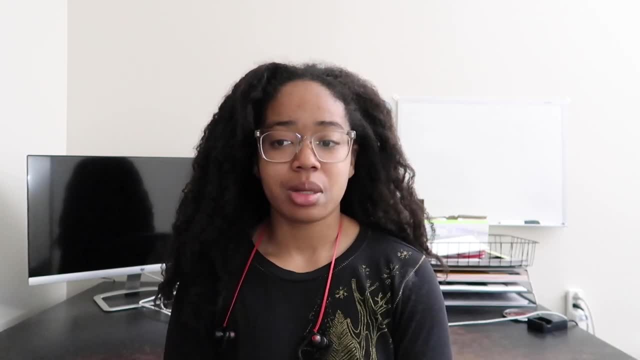 school and I knew that I wanted to do something involving machine learning and electrical engineering. for medicine. I didn't really have a clinical focus, but I knew that I was interested in electrophysiological systems, so parts of the body that use electricity, and in most cases that's either the heart or 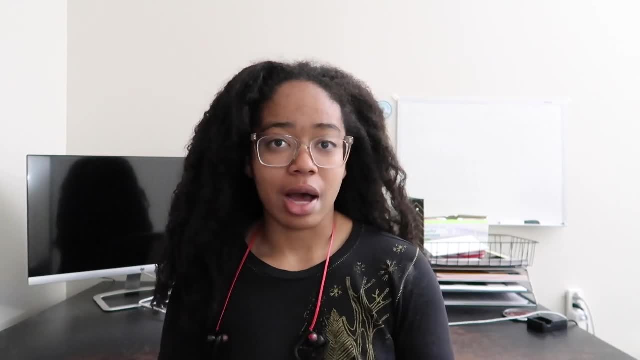 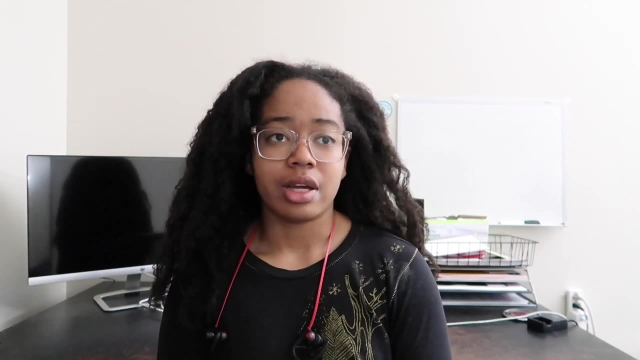 the brain. My program does rotations so you get to kind of try out labs before you commit. So my first rotation was fully in the media lab. I was working in a lab called camera culture. they find new ways to see things and that's like a really broad statement. but if you check out their